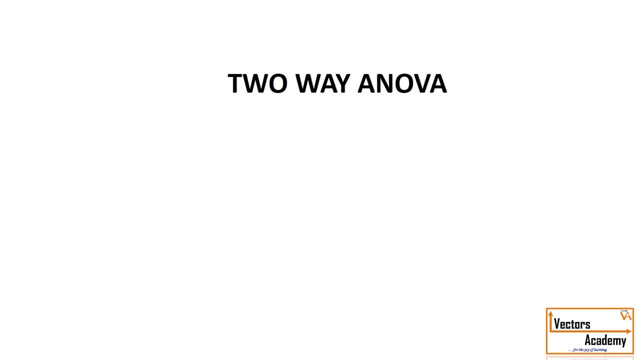 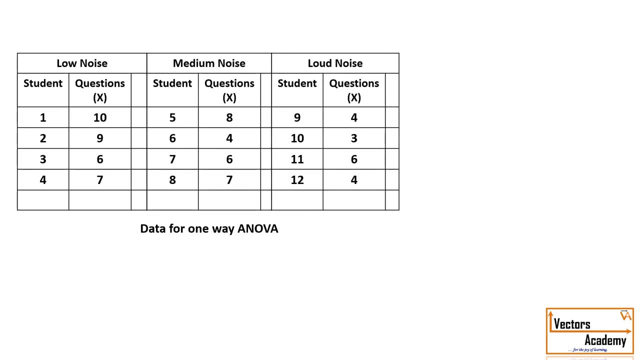 Now let us understand how to solve a two-way ANOVA. Now let us first have a look at the difference between a two-way ANOVA and a one-way ANOVA. In one-way ANOVA, the data given is like this: The noise is divided into three categories. 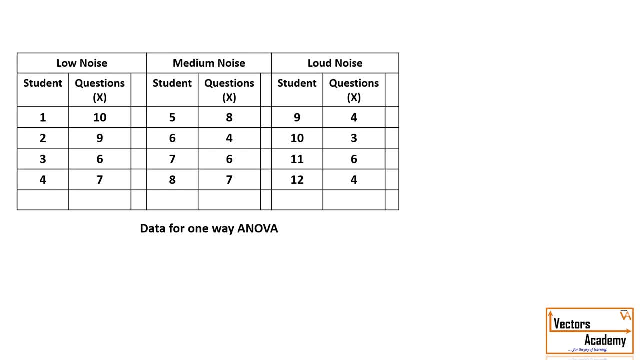 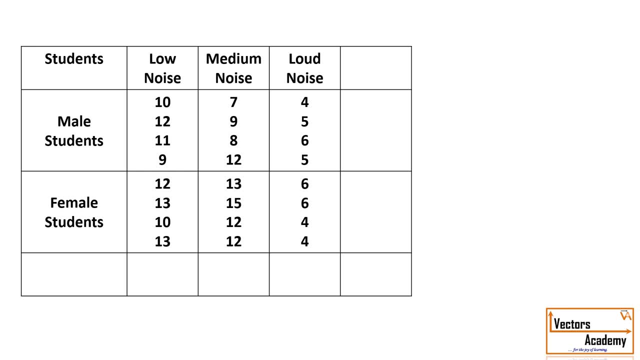 and the marks of the student in each category is noted, Whereas in the two-way ANOVA the noise is given in three categories, where the student as well are divided into two categories. So in this we need to study three major things. First, does the noise have an effect on the 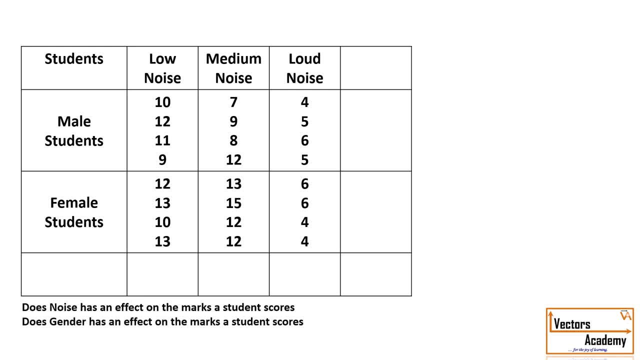 student marks. Does the gender of a student has an effect on the marks? And third, does the gender affect how the students react to the noise? So there are three different categories to be studied. One is the effect of noise on the marks. Second is the effect of gender on the marks. 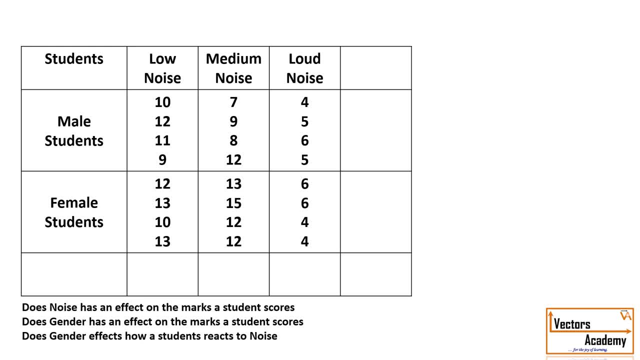 And third is the collective effect of gender and the noise on the marks. So let us start with first defining our null hypothesis. Our null hypothesis can be defined as there is no effect of one variable on the another. Now we will start with our calculation. 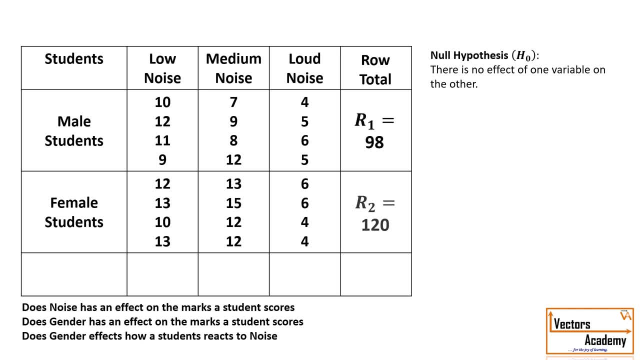 First of all, we need to have the row total as well as the column total. Once we have that, we can move further to calculate the correction factor. Just as in the case of one-way ANOVA, the correction factor is given by the square. 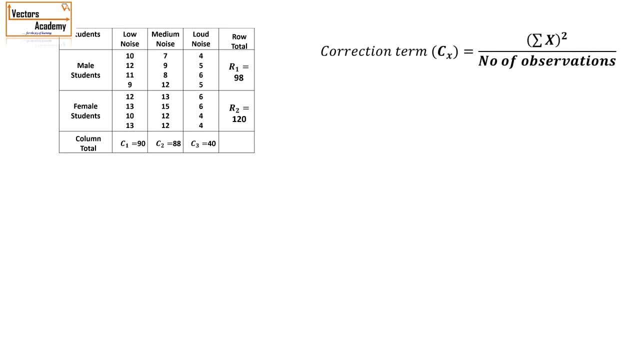 of the summation of all the given readings divided by number of observations. So that will come to 1980.. Now, secondly, we need the sum of squares of total. So we need to square all the individual marks and subtract it from the correction factor. Then we have sum of squares. 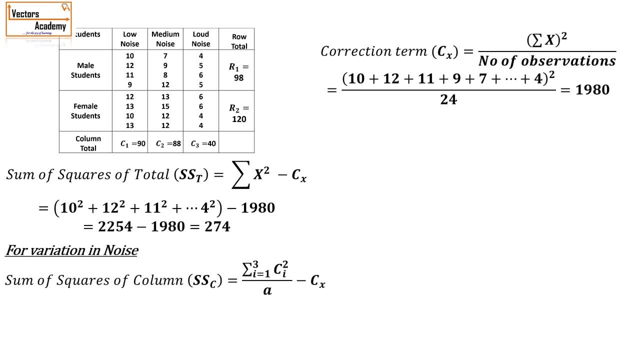 of the columns. We have already found out the column totals right, So we need to square them and add them. divided by number of readings in each column, You can see each column contains 8 readings, So we divide it by 8 and minus the correction factor, That gives you 200.. 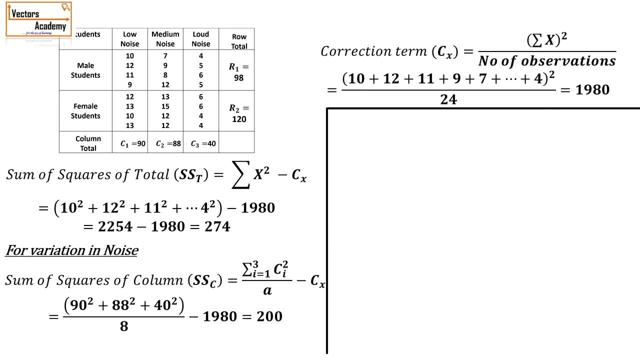 Next we need to find the sum of squares of the rows. Now we have already made row totals as well. So 98 square plus 120 square divided by number of readings in a row, That is, you can see there are 12 different readings in one row, right? So we divide it by: 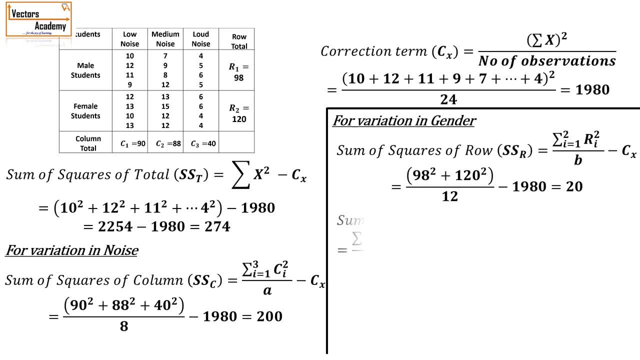 12 minus the correction factor, That gives you 20.. The next comes sum of squares within groups. Now there are six different groups which are formed: Male students with low, medium and loud noise, and female students with low, medium and loud noise. So we need to find the 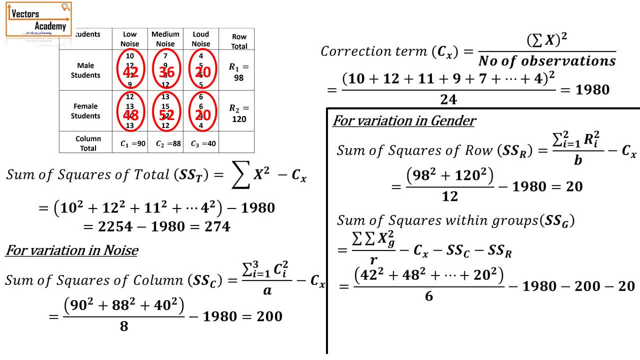 total of each group, square them and add them, divided by number of groups, That is 6 minus the correction factor and minus the previous totals which we have made. That is sum of squares of column and sum of squares of rows. So that will come to 16.33.. 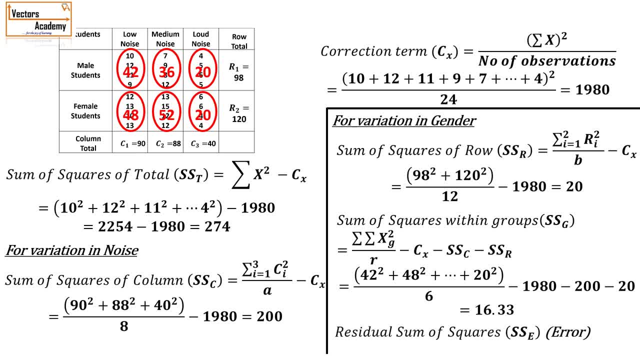 Next is the residual sum of squares, which is important to find out, the F-ratio. So that is found out by sum of squares of total minus all the sum of squares which we have found out. So that comes to 37.. Now we will make a table of all the data which we have found out so far. 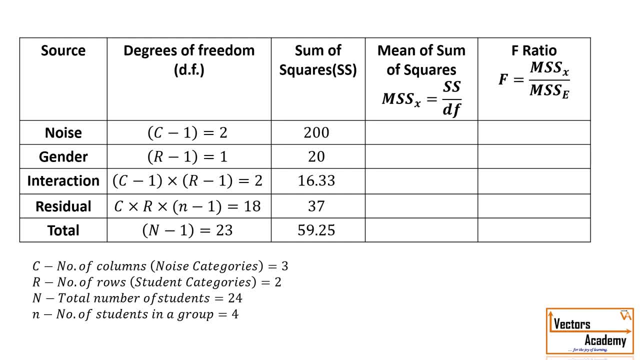 Have a careful look at how the data is being calculated. So we have found out that degrees of freedoms are found out For the noise. we had three columns, So number of columns minus one gives the degrees of freedom for the noise, For the gender we had. 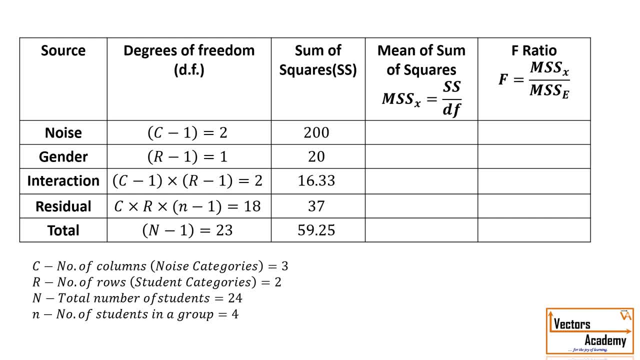 two columns, male and female, Minus one, that gives you one. The interaction between the noise and the gender. that is found out by number of columns minus one into number of rows minus one. That comes out to two: The residual and the total. 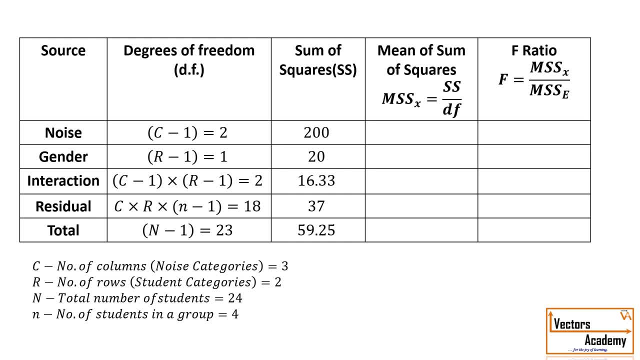 To find out the mean sum of squares, we have to divide the sum of squares by degrees of freedom. So we will get the respective values of mean of sum of squares. Now the F-ratio, Now the F-ratio for all. the mean sum of squares is calculated by the respective 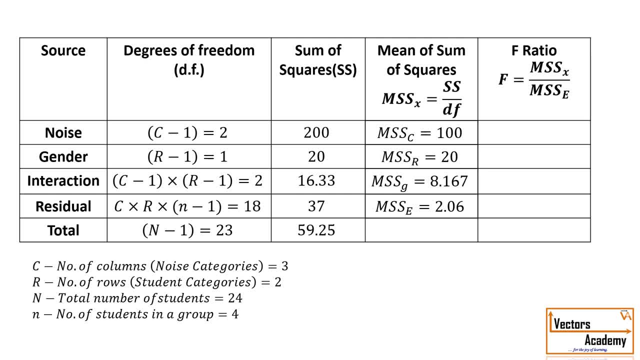 means divided by the mean sum of squares of the residual quantity or the error. So 100 divided by 2.06.. That gives you 40. So we have got 40.73.. 20 divided by 2.06, that is 9.81.. And 8.167 divided by 2.06, that gives you 3.97..